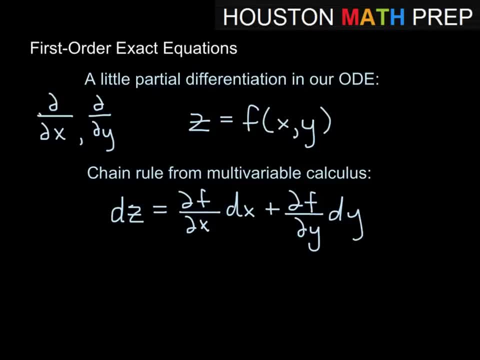 And that will be our differential for z. So just doing A little bit of abbreviating here, I'm going to go ahead and call this partial derivative of f with respect to x. I'm going to call that capital M here. So you just want to remember that M is actually a function of x and y, perhaps. 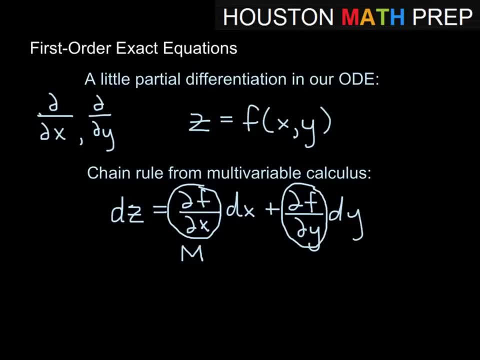 And then our partial derivative with respect to y, I'm going to call that capital N. Those are pretty standard notations there And again, remember, N is some function right, involving perhaps x and or y. So the idea for our differential 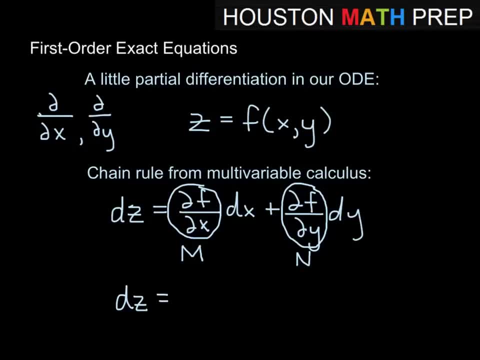 Differential, in other words dz. the shorter way we might see it would be M dx plus N dy, And so if you've had any course like multivariable calculus- maybe a calculus 3 or something where you talked about vector fields and gradients and potential functions, a lot of the math that you'll do in solving exact equations will be very similar to the ideas that you talked about. maybe with those things. 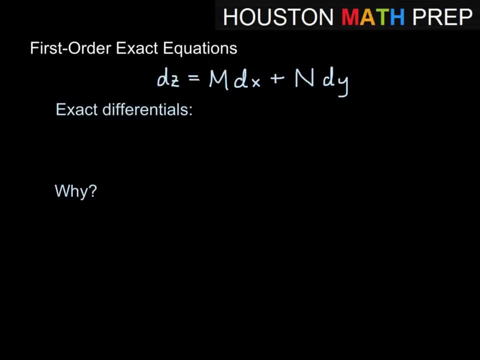 So this differential dz, then, is going to be what we call an exact differential, given that the following is true: Given that the partial derivative of M with respect to y is equal to the partial derivative of N with respect to x, And the reason why that is, if any of you have studied, 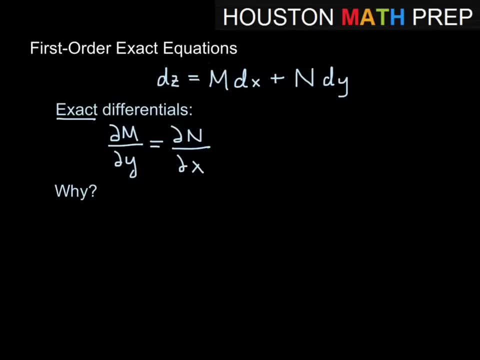 Partial differentiation. you know, if we have a well-behaved function, in other words it's continuous and it also has continuous first partials- then we're told that both the mixed partial second derivatives should be equal to each other. In other words, this expression that I'm writing here, the second partial derivative of F with respect to x, then y, and then also y then x. those should be equal to each other. 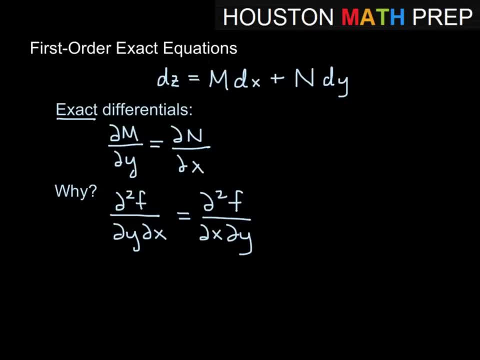 So just real quickly, why that gives us that. this means we have an exact differential, if we take a look, and we start here. so in other words, the second derivative of F with respect to x and then respect to y. remember, on the bottom there we read from right to left. so that's with respect to x, then with respect to y. 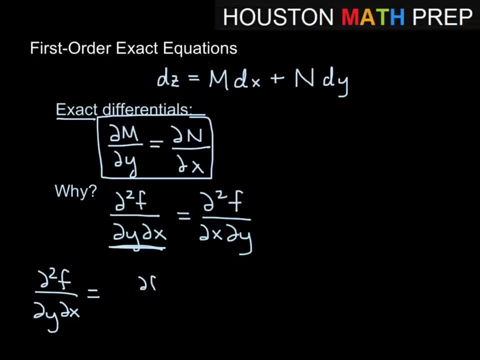 So, in other words, we're looking at the partial derivative with respect to x And then we are from that. we are then taking the derivative with respect to y And- remember, just a second ago we said this thing in the parentheses- we're calling M. so, in other words, this is the partial derivative with respect to y of M, which gives us the left side here. 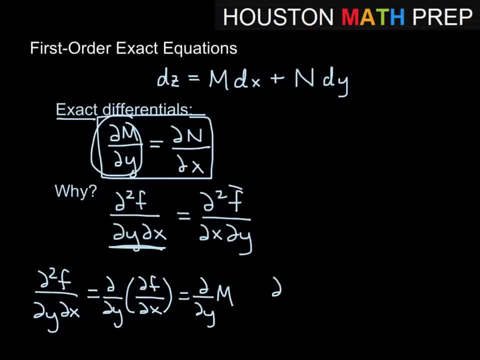 And then if you look at the other piece, if we look at this, half the partial derivative with respect to F, First y, then of x. the idea there is, we're taking the derivative with respect to y first, then, whatever we get there, we're taking the partial with respect to x. 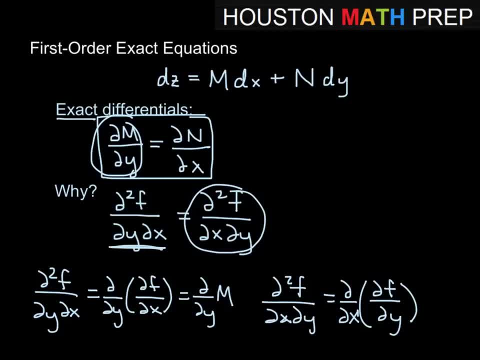 And we said this partial F with respect to y was N, right. So this is the partial with respect to x of N, which gives us this half here. So this is the condition. So we're giving a moment that we wanna check. 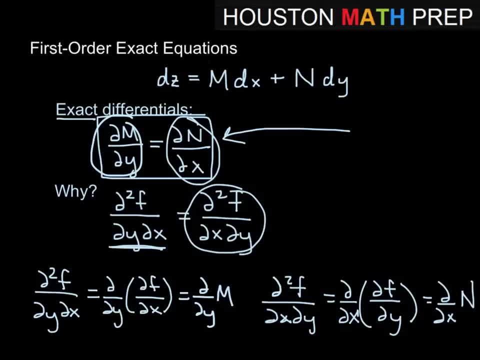 And if we have this being true, then we have an exact differential. in other words, we have an exact equation and we're gonna show you how to work with that to find solutions to these equations. All right, so we've got a few examples here. so the first one: we're just checking for exactness. 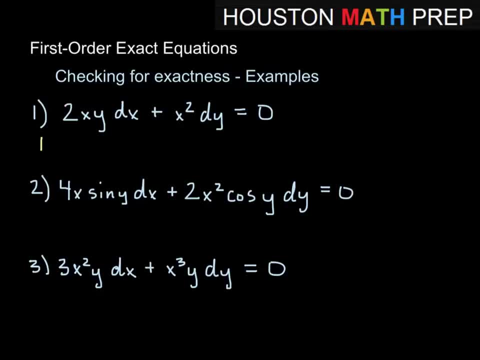 2xy dx plus x square dy equal zero. so our M for the first one is equal to 2xy Zx equal 2, and the answer has no formula if we're even out. Zx equal 2, and the answer has no formula if we're even out. 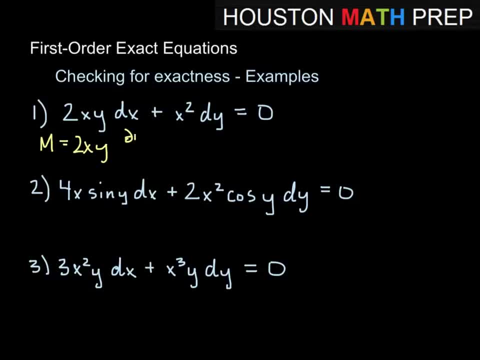 Zx equal 2, and the answer has no formula. if we're even out And remember that's what these two hartrega functions do, These two hartrega functions do These two hartrega functions do, And remember we're taking the partial derivative of m with respect to y. 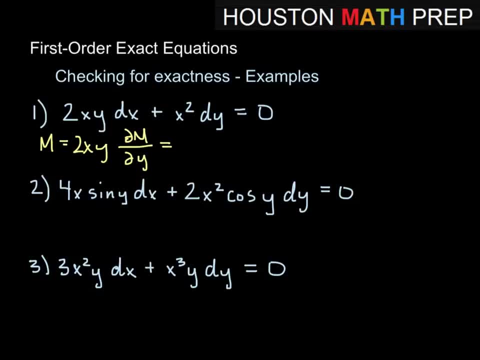 So, treating x as a constant, 2x is basically your constant Derivative with respect to y would be 1, so you'd get 2x times 1.. So 2x is our derivative of m with respect to y. 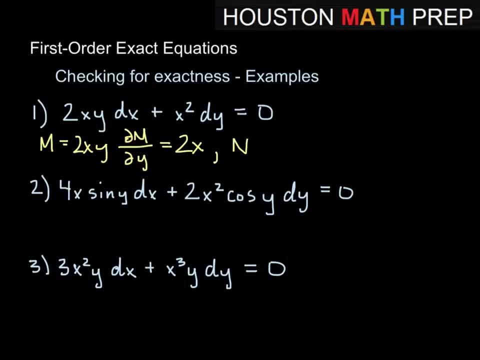 And then if we look at n, which is x squared, then the partial of n with respect to x. so we have no constants there and we look at that as just being 2x. So these are the same, which means this one is exact here. 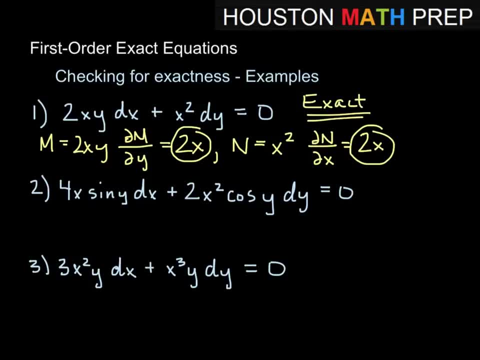 And so we would then follow the steps to solve the equation, which we'll get to in just a minute. All right, next one, number 2.. Here we have our m is 4x sine y. So when we take the partial derivative of m with respect to y, 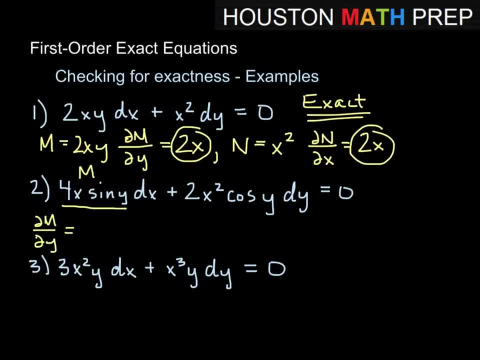 that means we treat 4x as a constant out front of our sine y. So the derivative of the sine y part would give us cosine y. So that gives us 4x cosine y for our partial of m with respect to y, And then the 2x squared cosine y is our n here in this example. 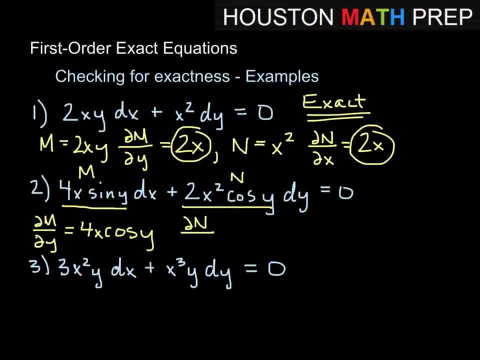 So when we take the partial of n with respect to x, so the cosine y, since there's no x in that, we treat that as a constant, So we'll ignore that right now It's a constant multiple. So derivative 2x squared would give us 4x. 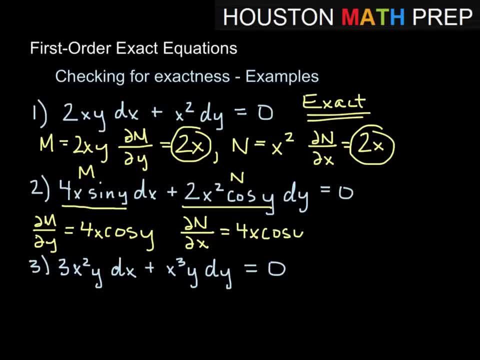 And then we'll include the cosine y as constant as well. So you can see that the derivative of 2x squared would give us 4x. And then we'll include the cosine y as constant as well. So you can see these match. 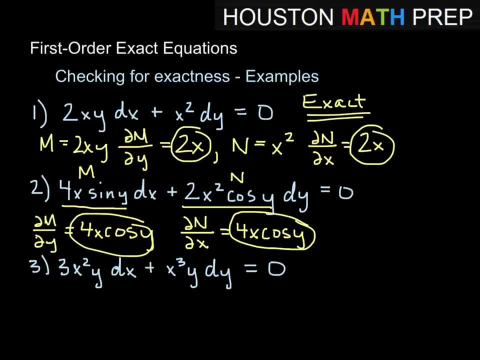 And so, since those match, it's exact. So this is an exact equation here, And we would then use the exact steps to solve which we're going to get to real quick. One more Here: in this one we have 3x squared y. 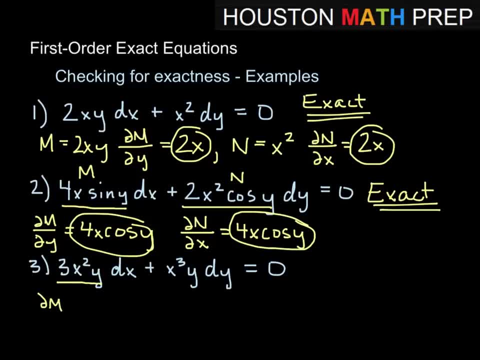 That's our m. So our partial of m with respect to y, 3x squared, is a constant Derivative of y, is 1.. So we get 3x squared, And then partial of n with respect to x. Now our n is x cubed y. 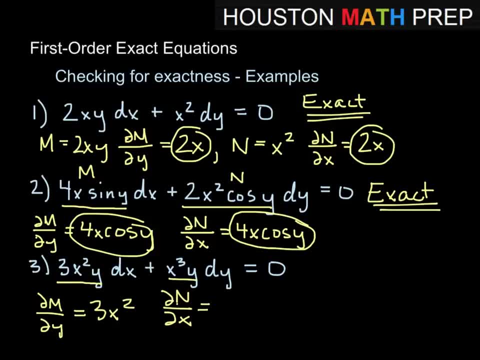 So we treat the y as a constant And then the derivative of the x cubed part would be 3x squared. So it would be 3x squared times y. So you notice these do not match. So this is not an exact equation. 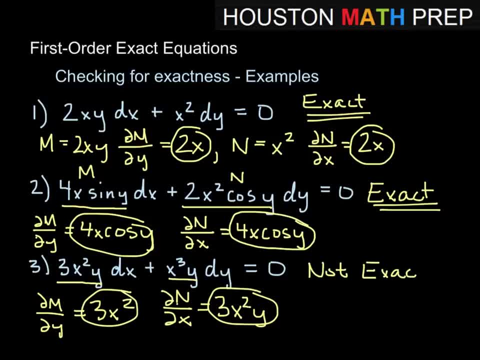 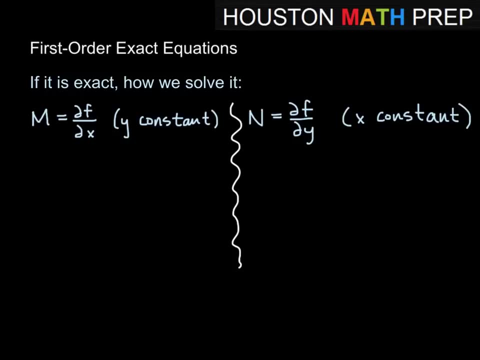 So we would have to find some other way of solving this, Either to make it exact by using, maybe, an integrating factor, or finding some other way to manipulate this, to solve. So, if we find that our equation is exact, and remember that m is the derivative of the function with respect to x, partial- 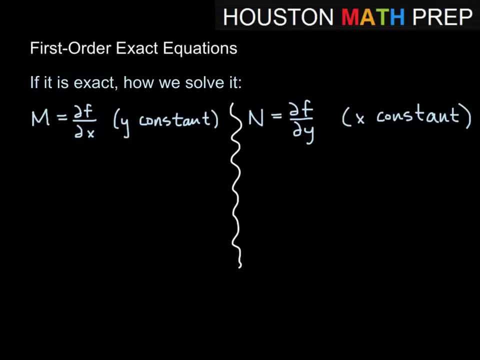 And then n is the partial with respect to y, of the function. So in each of those cases, treating the opposite variable as a constant. So what we want to do in terms of m, to get back to the original, is we would need to go back in terms of x. 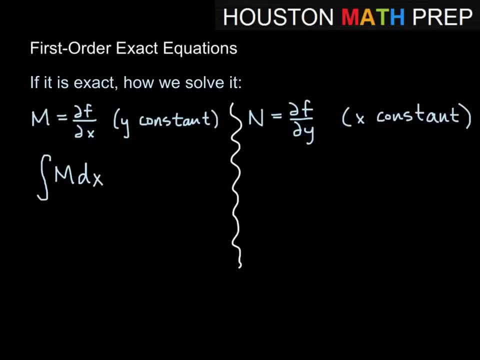 So we're going to antiderivative with respect to x And remember when we do that we'll end up with some sort of constant of integration that comes into play. Now y is a constant when we're working with m, So the thing we want to remember is that our constant 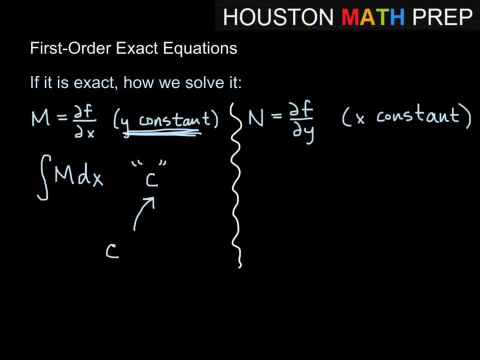 will actually probably be a function that we treat as a constant, And it will be in terms of y, because y is a constant. If we're working with n and trying to get back to the original f, then we will need to antiderivative in terms of y. 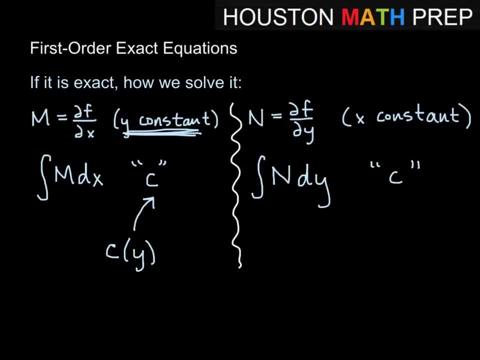 Again, we'll have some constant of integration when we do that over here as well. What we'll need to do, then, is remember that x is constant when we're dealing with n, So this constant of integration will actually likely be a function of x. 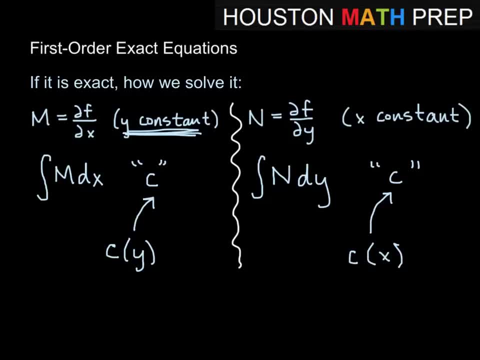 Different books and different sources will treat these. Some of them will call them f of y and g of x, or however they'll notate it. I'll just call this one c1 and I'll call this one c2.. And just remember that these are going to be functions. 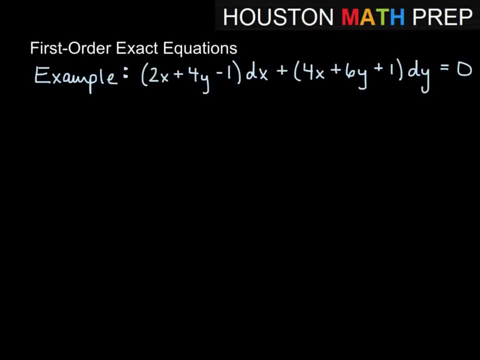 and not just some number that we're dealing with. Alright, we'll work out an entire example. So we have 2x plus 4y minus 1 quantity dx. So this is going to be our m Here Plus 4x plus 6y plus 1 dy. 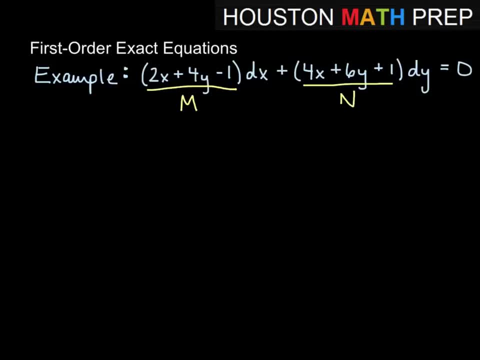 So our n is this quantity here, And so first we want to check exactness, So we'll check exactness first. Okay, so partial derivative of m with respect to y. The first term does not have y in it, so it's a constant. 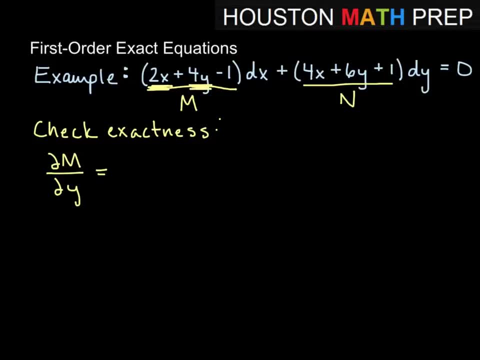 So we get 0 out of that. The next term derivative of 4y with respect to y is 4.. And then minus 1 is a constant, so we get 0 out of that. So our partial of m with respect to y is 4.. 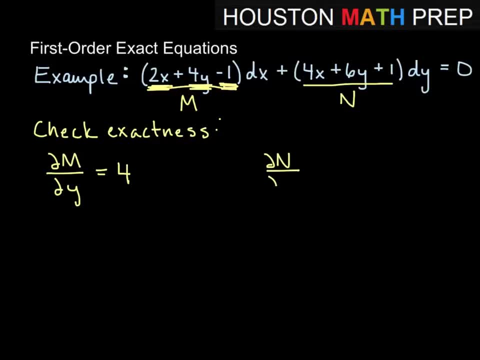 Then the partial derivative of n with respect to x, So derivative of 4x with respect to x, is 4.. And then 6y is a constant, because we're treating x as our variable And 1 is a constant. And 1 is a constant also. 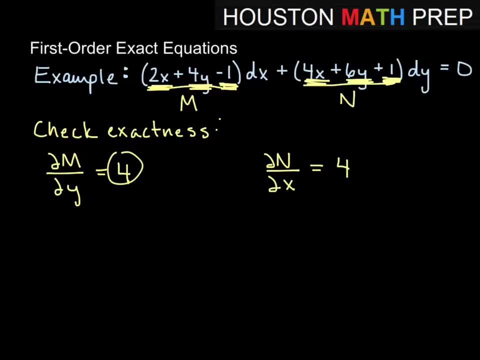 So both of those terms will give us 0. So you can see these match certainly. So they are giving us that this is an exact equation. We have exactness, And now what we'll do is then take the antiderivative with respect to the appropriate variables. 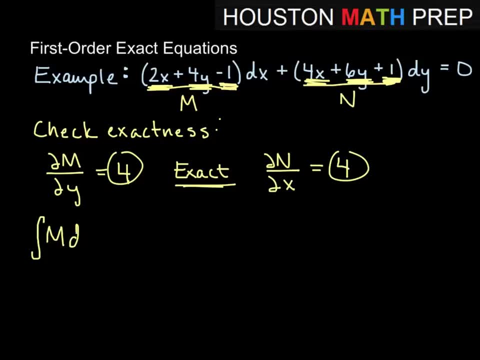 So we will antiderivative of m in terms of x And that will give us So the first term, 2x: Integrate, we get x square. If we integrate 4y with respect to x, that gives us 4xy. 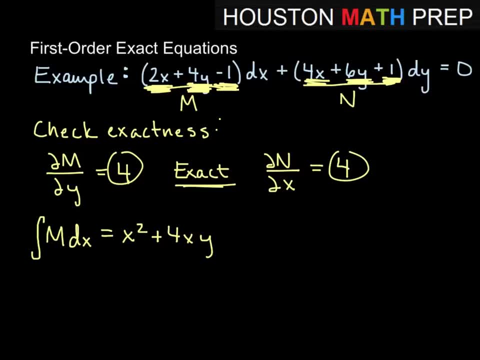 And if we integrate a minus 1 with respect to x, that gives us minus x. And then remember, our constant of integration we may get would be in terms of y there, And I'll call this c1. So we might have some what we are treating as constant terms in terms of x. 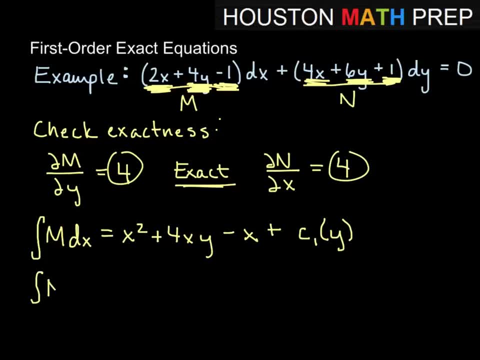 But they have y in them And then antiderivative of n with respect to y. Alright, so we're integrating 4x with respect to y gives us 4xy. If we are integrating 6y with respect to y, that will give us 3y square.